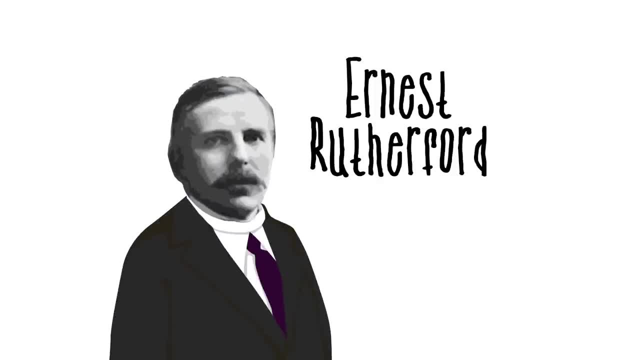 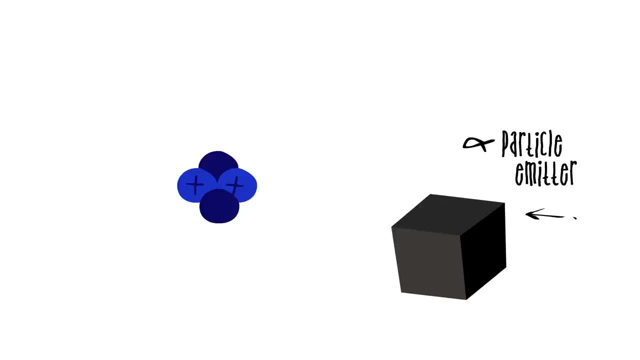 The next puzzle piece came from Ernest Rutherford in England In 1909, Ernest Marsden and Hans Geiger, working for Rutherford, shot alpha particles at gold atoms and were stunned to find that some bounced straight backwards. This showed that most of the mass of the atom is concentrated in a tiny nucleus. 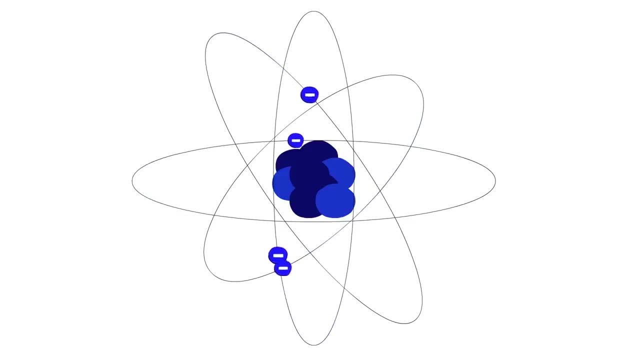 The cartoon atom you learn in grade school, with electrons orbiting like a miniature solar system. That's Rutherford's. There's one little problem with Rutherford's atom: It can't work. Classical physics tells us that an electron whipping around in a circle emits light. 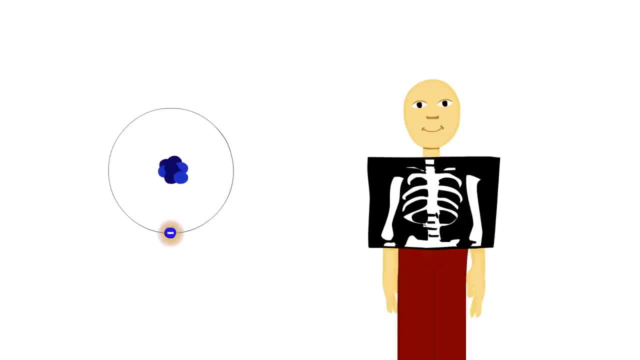 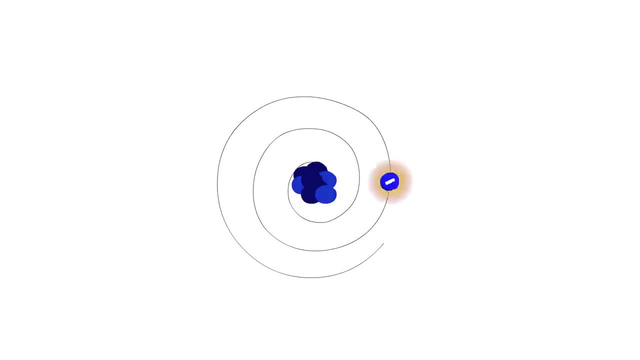 and we use this all the time to generate radio waves and X-rays. Rutherford's atom should spray X-rays in all directions for a brief instant before the electron spirals in to crash into the nucleus. But Niels Bohr, a Danish theoretical physicist working with Rutherford, 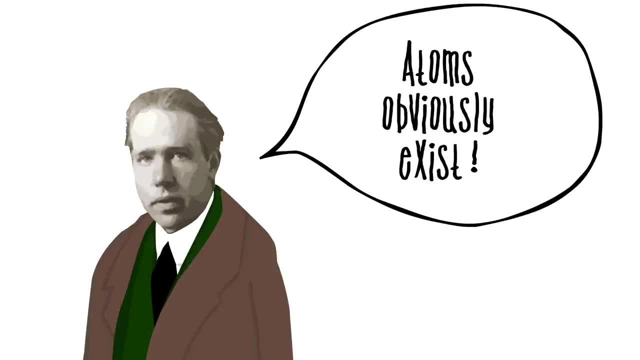 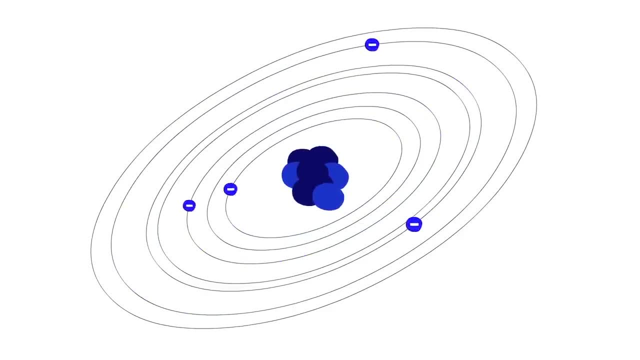 pointed out that atoms obviously exist, so maybe the rules of physics needed to change. Bohr proposed that an electron in certain special orbits doesn't emit any light at all. Atoms absorb and emit light only when electrons change orbits and the frequency of light depends on the energy difference. 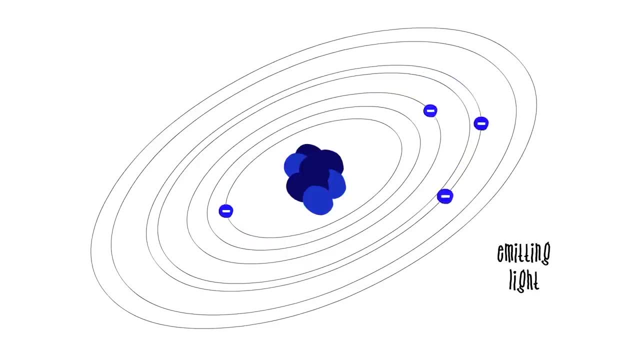 in just the way Planck and Einstein introduced. Bohr's atom fixes Rutherford's problem and explains why atoms emit only very specific colors of light. Each element has its own special orbits and thus its own unique set of frequencies. The Bohr model has one tiny problem. 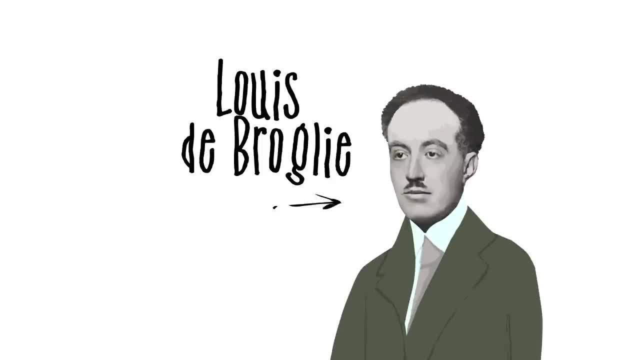 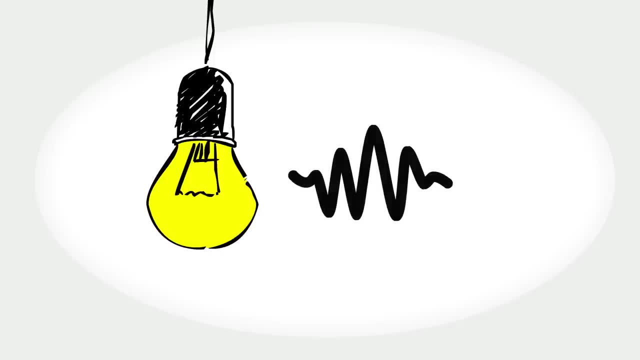 There's no reason for those orbits to be special. But Louis de Broglie, a French PhD student, brought everything full circle. He pointed out that if light, which everyone knew is a wave, behaves like a particle, maybe the electron, which everyone knew is a particle. 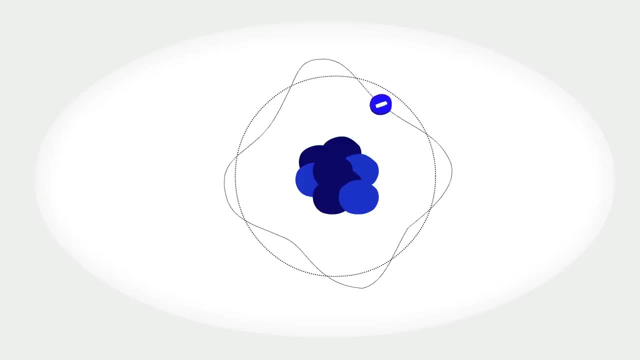 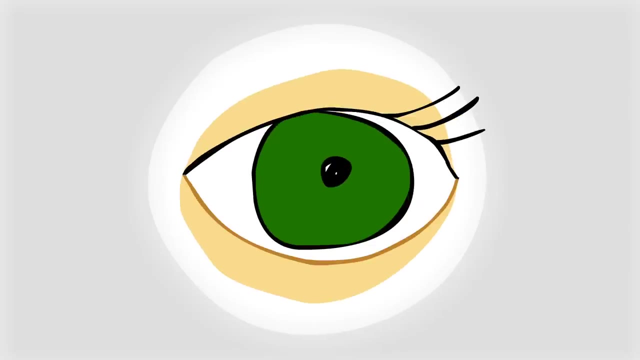 behaves like a wave. And if electrons are waves, it's easy to explain Bohr's rule for picking out the special orbits. Once you have the idea that electrons behave like waves, you can go look for it And within a few years. 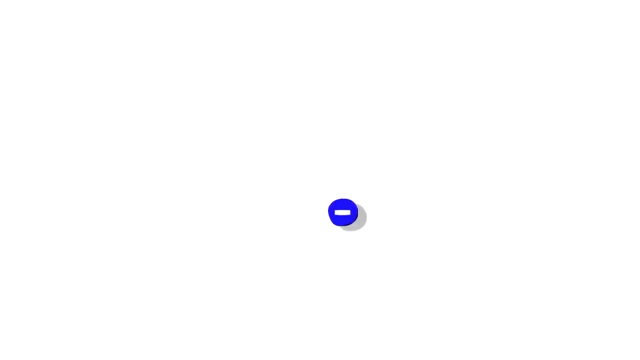 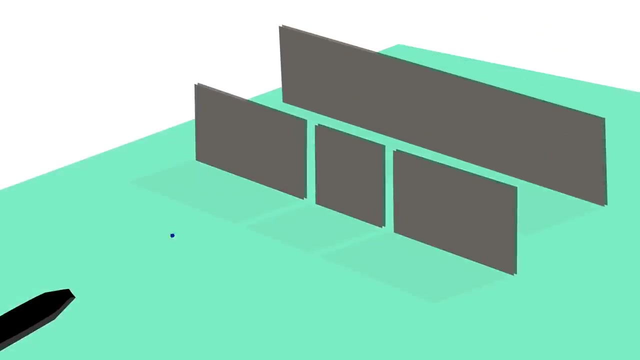 scientists in the US and UK had observed wave behavior from electrons. These days we have a wonderfully clear demonstration of this shooting single electrons at a barrier with slits cut in it. Each electron is detected at a specific place at a specific time.